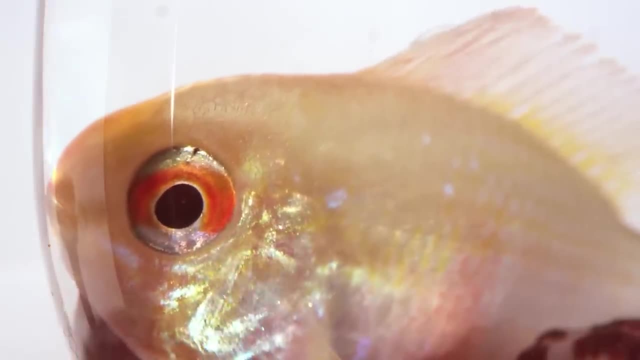 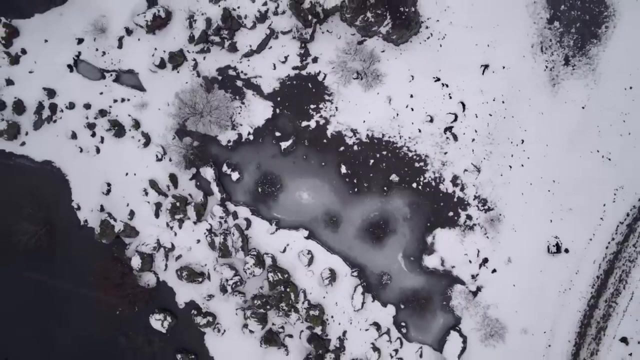 Fish are cold-blooded, which means their body temperature is the same as the environment where they live. If they live in the freezing waters of the Arctic, their bodies adapt to that cold temperature, And if they live in a tropical location where the water is much warmer. 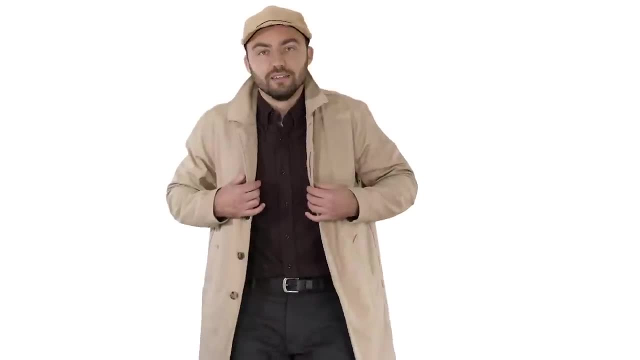 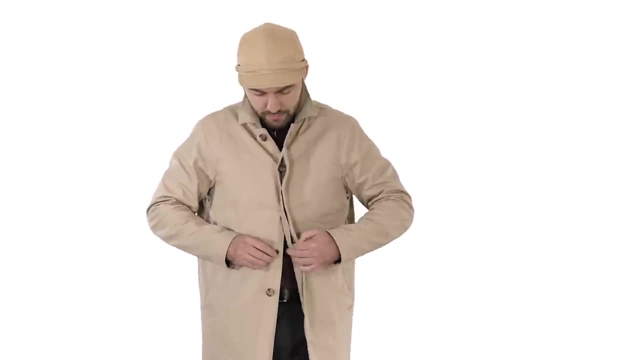 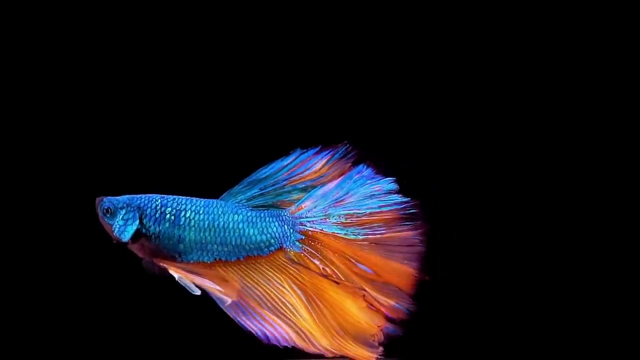 their bodies adapt to live there too. Humans are warm-blooded. This means regardless of whether it's very cold or very hot around you, your body temperature always stays the same, unless you have a fever. Fish come in a wide variety of colors, sizes and characteristics. 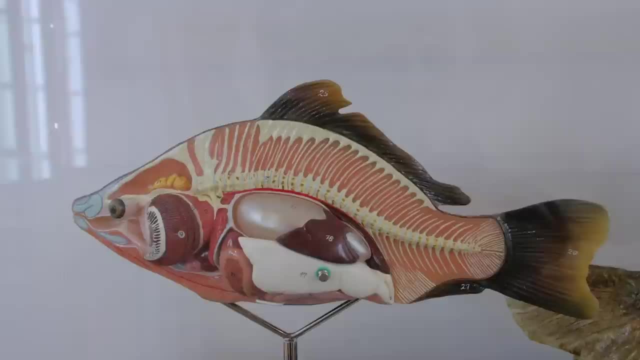 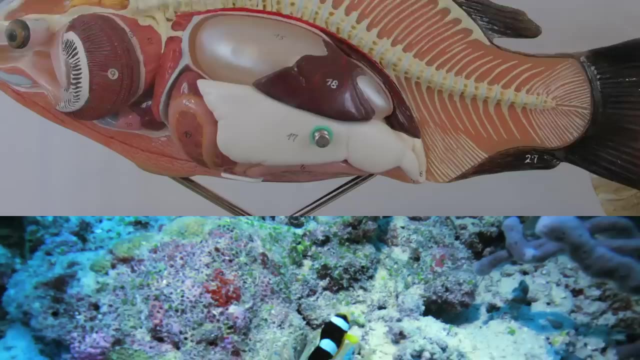 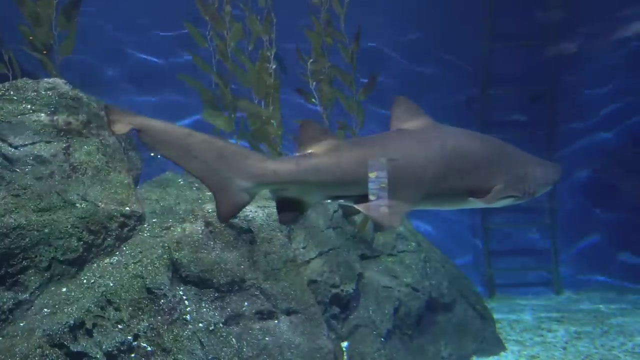 But all fish have certain things in common. For one thing, they are vertebrates, which means they have backbones. just like humans, Fish also have fins that help them move and swim through the water. Their back fin helps push them forward, while the fins on each 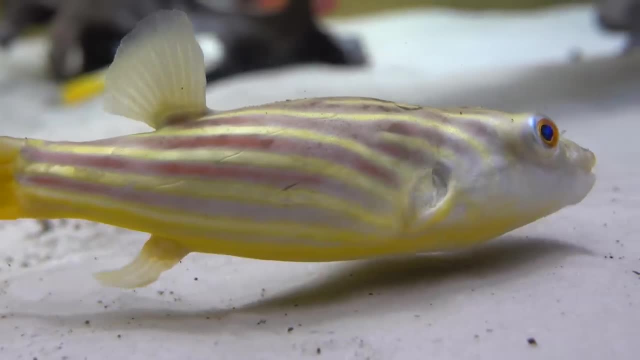 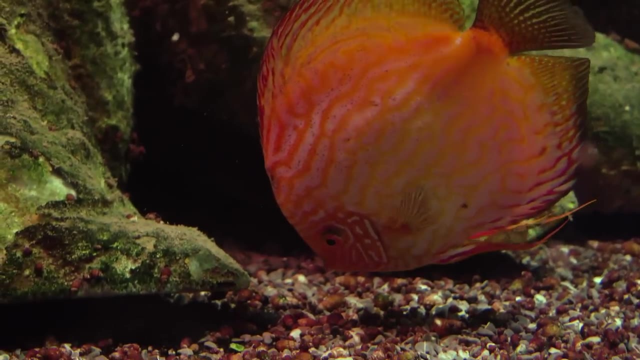 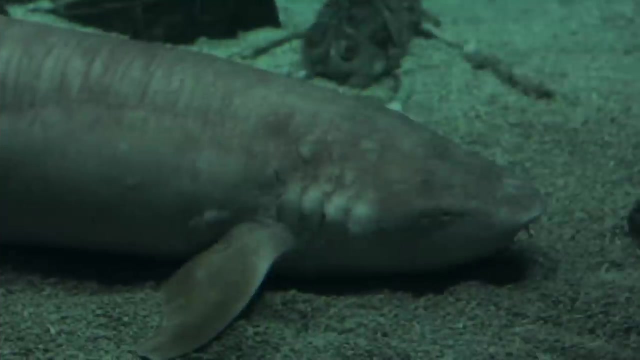 side help them steer. Some fish have fins on the top and bottom of their bodies. Those fins help them stay in place and keep them from rolling over. Another characteristic of a fish is gills. You use your lungs to breathe air, But fish use their gills. The gills allow fish to breathe in water. Fish get their oxygen from their stomachs. Fish breathe water from their stomachs and airから в their sanitarium. Gills breath out oxygen and get their blood into their bodies. When they're opened they're engulfed with their body hair, but their stomach actually tightens, so water's all over the surface. 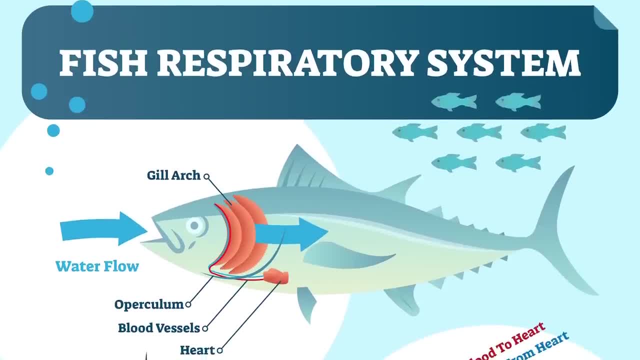 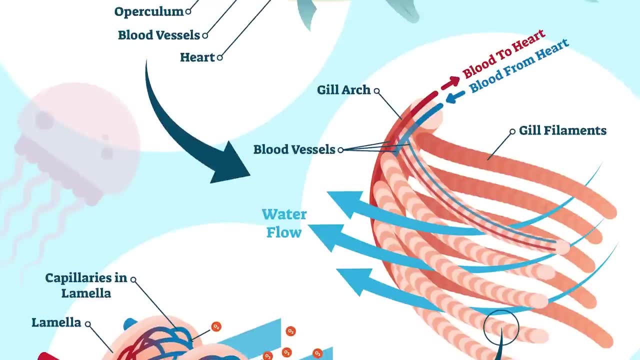 Every time the fish's lungs get smaller, small volumes of oxygen, of YES, are entwined into its slow from the water instead of the air. When water enters a fish's mouth, it passes through its gills. Little fibers in the gills absorb oxygen from the water. 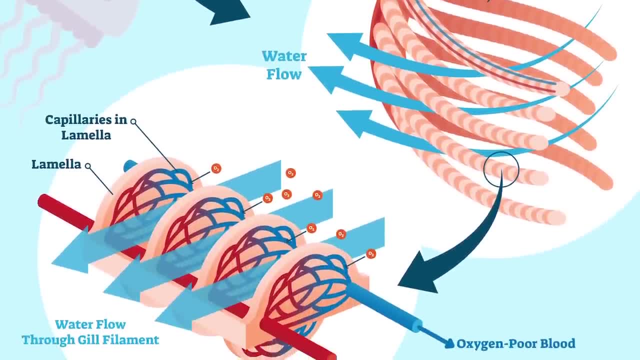 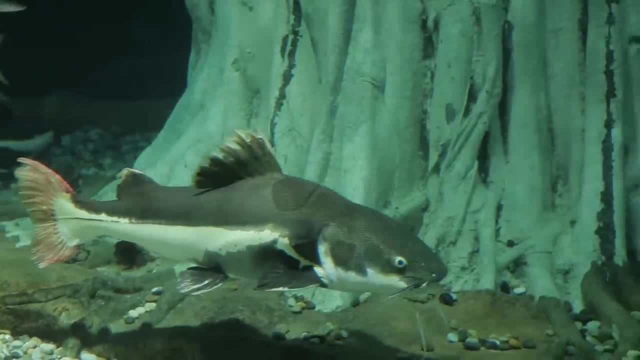 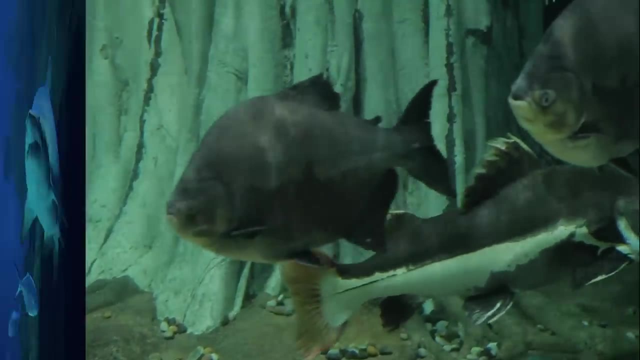 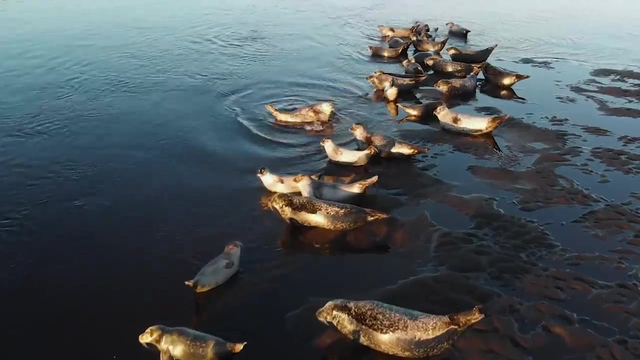 and move it into the fish's bloodstream. The heart then pumps the blood to move the oxygen throughout the fish's body. A fish's diet varies. Some fish, like catfish, eat plant life in the water or algae scraped off rocks, While fish like sharks eat other fish, as well as some mammals like seals and sea lions. 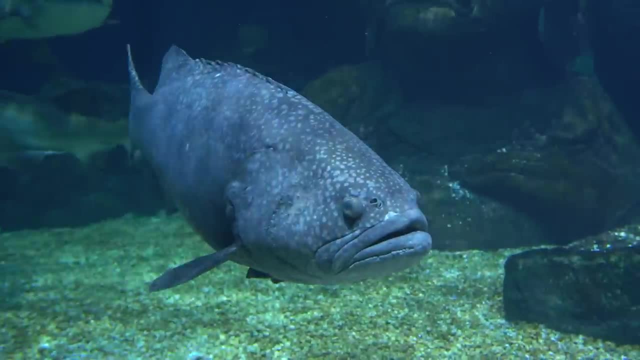 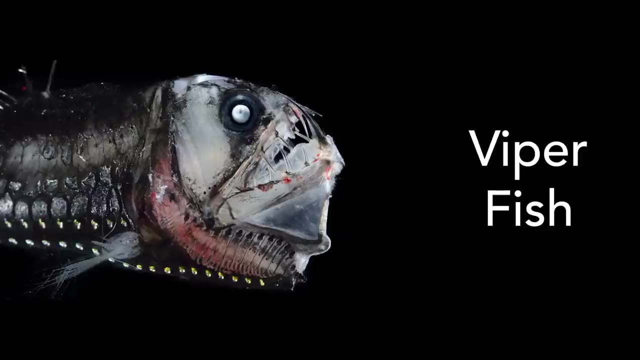 The larger a fish's mouth, the bigger the prey a fish can eat. The lanternfish and the viperfish both eat near the bottom of a body of water. The viperfish has fangs that are so large they can't even fit in its mouth. 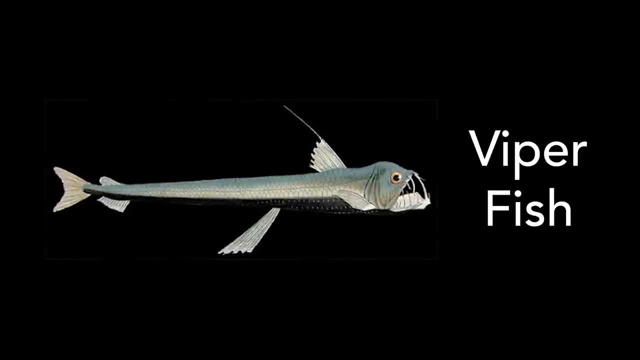 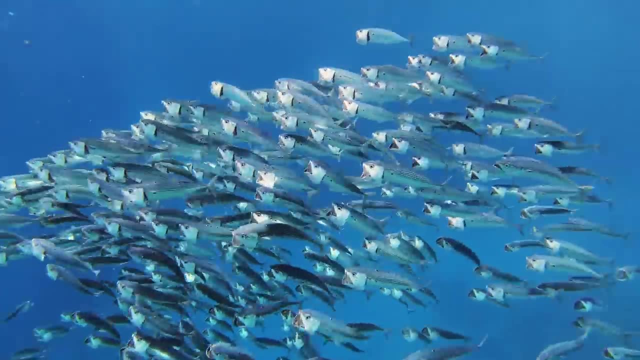 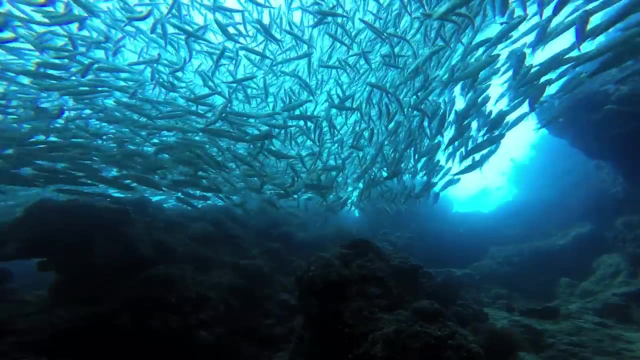 It also has a large dorsal spine that lights up to attract fish. Similar to a fishing lure, the herring and the mackerel both feed near the surface of the water. Their small mouths are good for eating smaller fish. For protection, many fish travel in a group called a school. 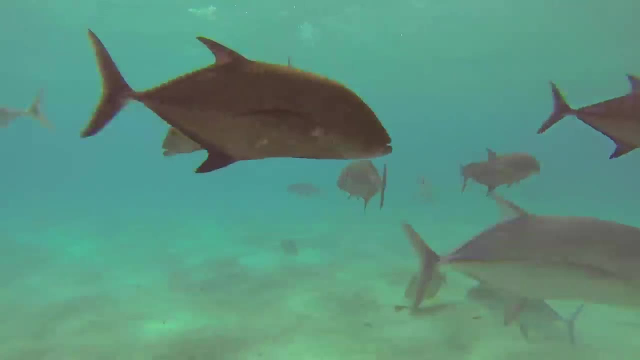 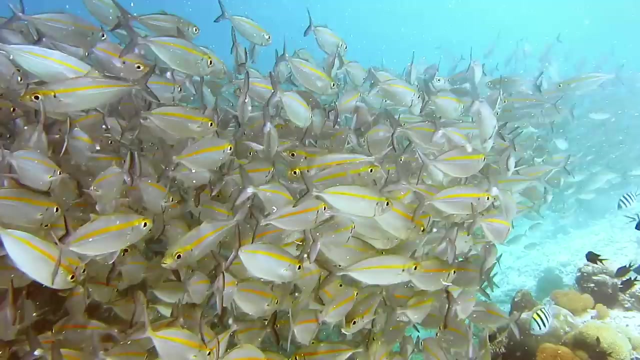 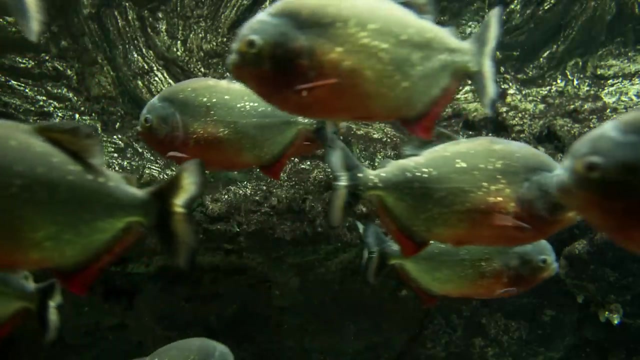 In a school. the fish swim close to each other. This makes them harder to catch, because a predator sees one large fish instead of many little fish. Most fish also have scales covering their mouths. The scales protect the skin from attacks. They also help the fish swim faster through the water. 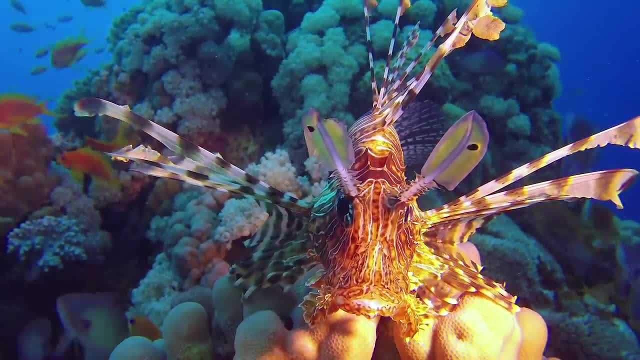 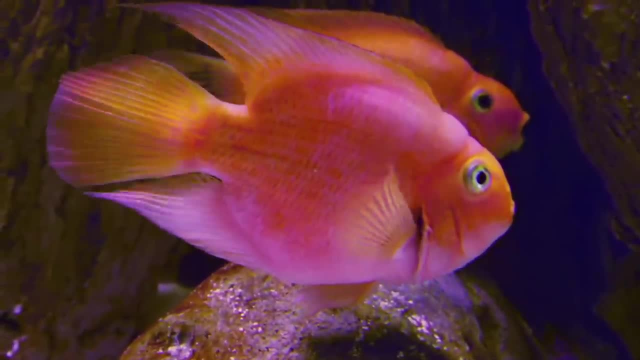 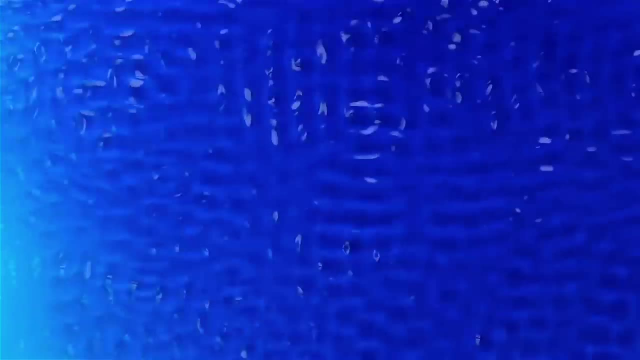 Did you know that fish have ears? Both humans and fish use their ears for balance. However, a fish's ears are not on the outside like yours are. Their ears are inside their bodies and are used to detect vibrations in the water. The eyes of a fish are similar. 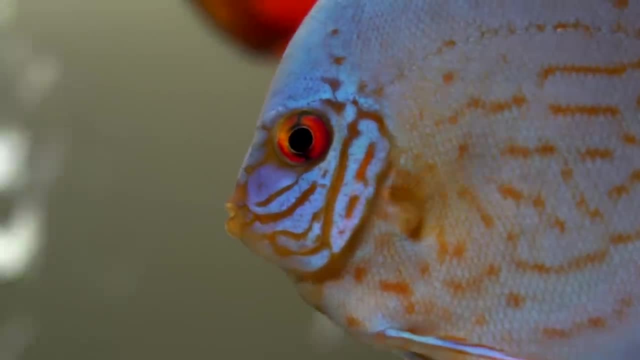 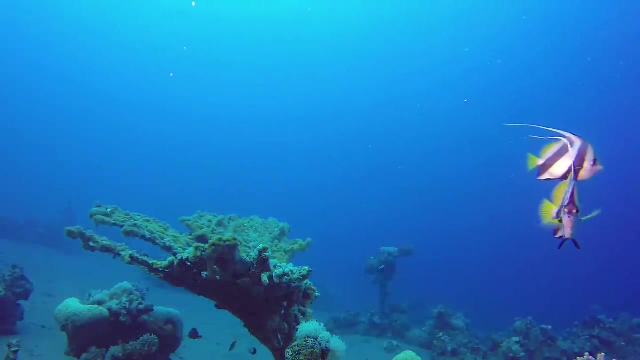 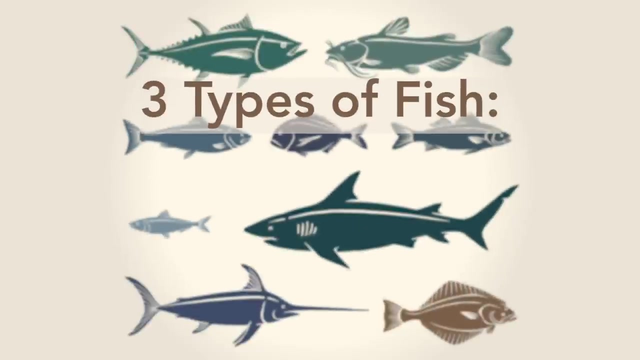 They can see color like you can. Their eyes are also used to communicate. The male fish uses his eyes to attract female fish. Fish have a sharp sense of smell and can detect odors in the water. There are three different classes or types of fish. 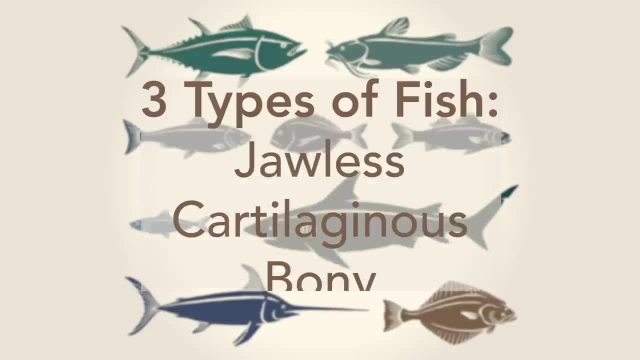 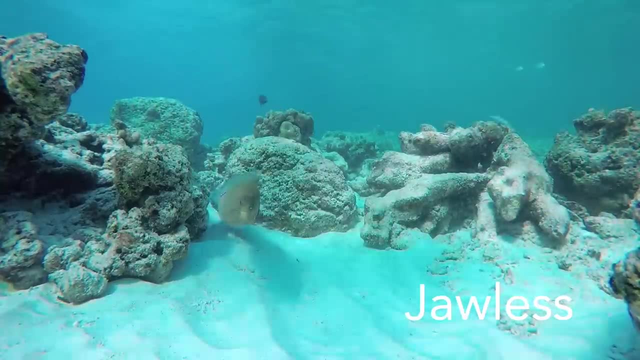 Jawless, cartilaginous and bony. Jawless fish do not have jaws, a stomach or a mouth. Jawless fish do not have jaws, a stomach or a mouth. Their skeletons are made up of cartilage instead of bones. 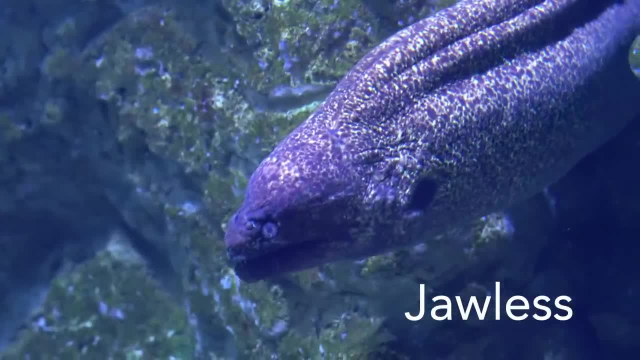 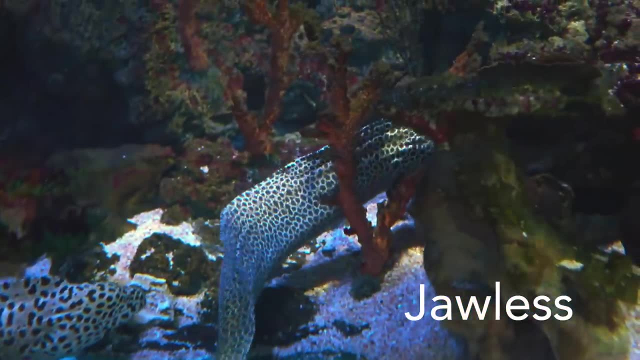 Most don't have fins on the sides of their bodies. Instead, they have a dorsal or caudal fin. Dorsal fins are on the middle of a fish's back, while the caudal fin is the back of the fish. 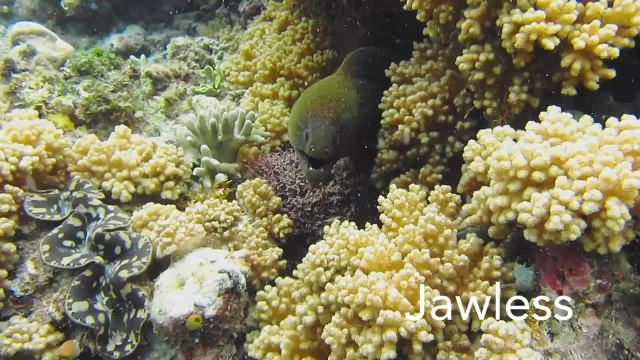 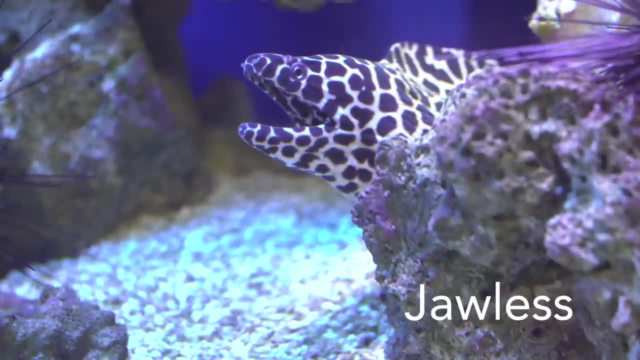 Jawless fish usually have long bodies. One type of jawless fish is called an eel. There are about 800 species of eels, 1,000 fauna and predatory species. They are long in length, from 2 inches to 13 feet. 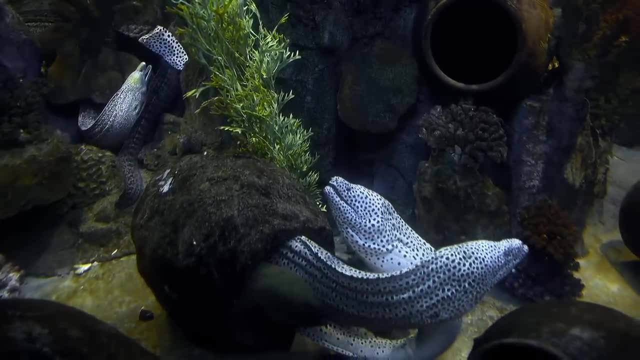 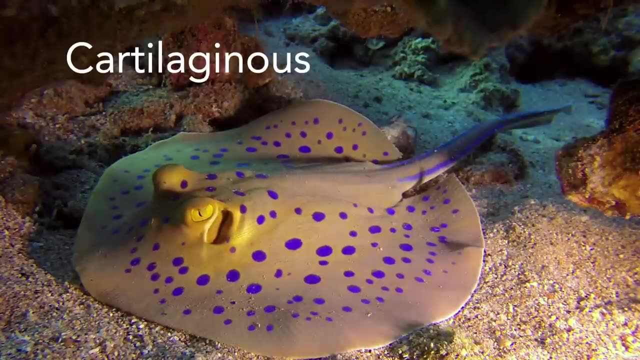 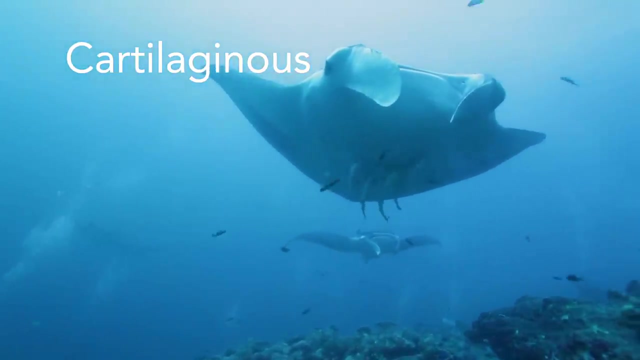 Most eels live in the ocean and can swim backwards. Cartilaginous fish have jaws as well as paired fins. They also have skeletons that are made of cartilage instead of bone. Just like jawless fish, cartilaginous fish are covered with a tough outer skin. 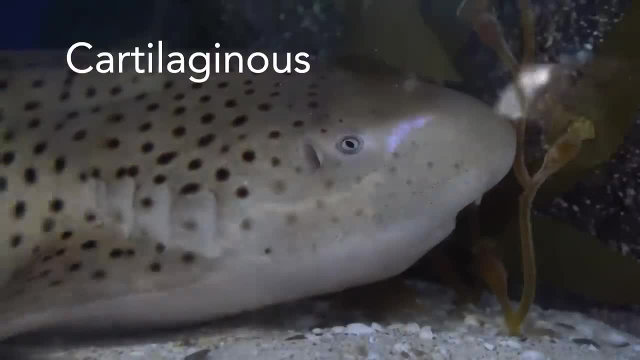 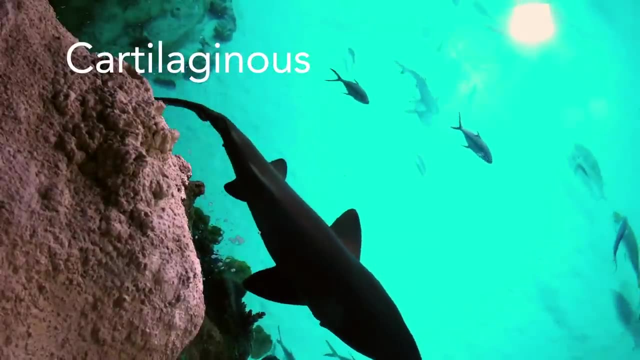 that includes placoid scales 1, différentes corotas gigantes umbora, alb Plana, mentioned in the article, with frecklings and abomas. They have five to seven gill slits as well as two nostrils. Sharks fall into this category, Even though the skin of a shark appears to be smooth. 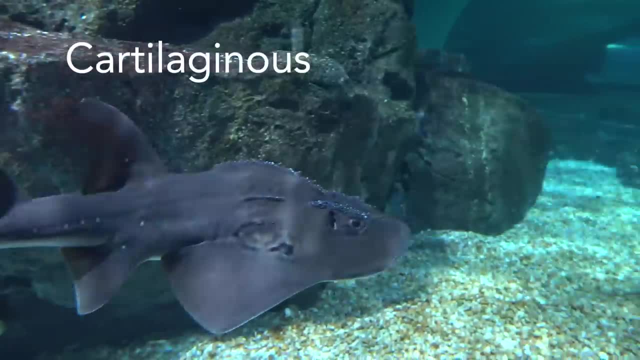 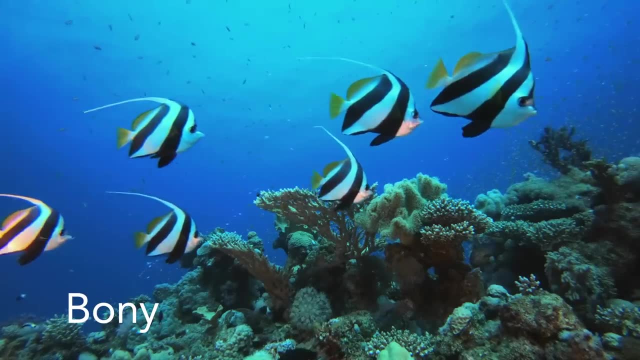 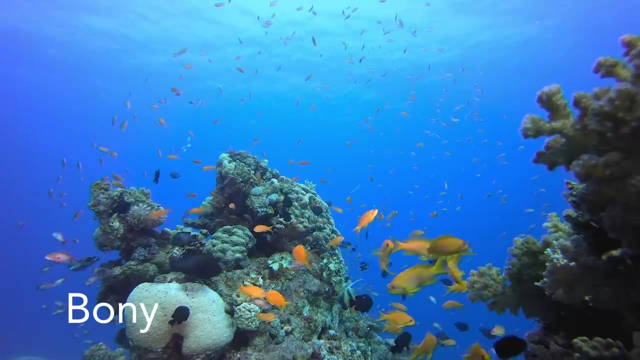 they are actually covered with scales that can be seen under a microscope. Bony fish have skeletons that are made of bone instead of cartilage. These fish have scales as well as a single pair of gill openings. This category is the largest class of fish, with over 20,000 species. 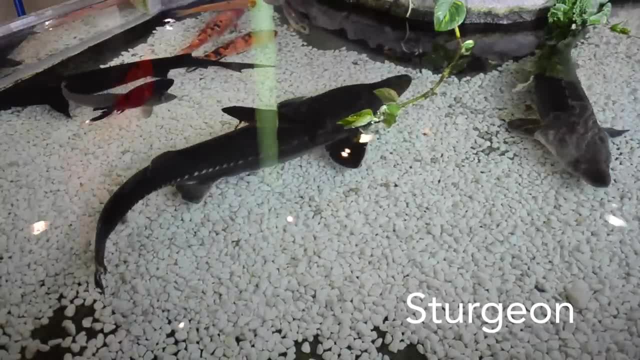 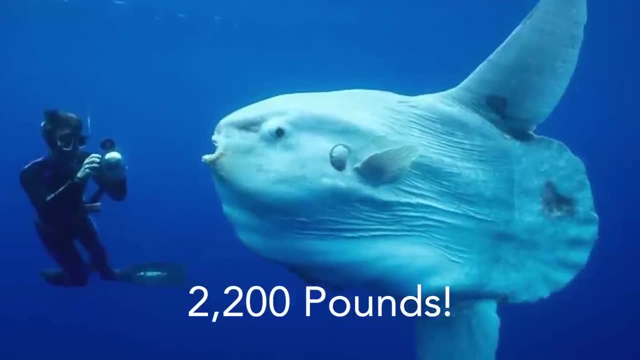 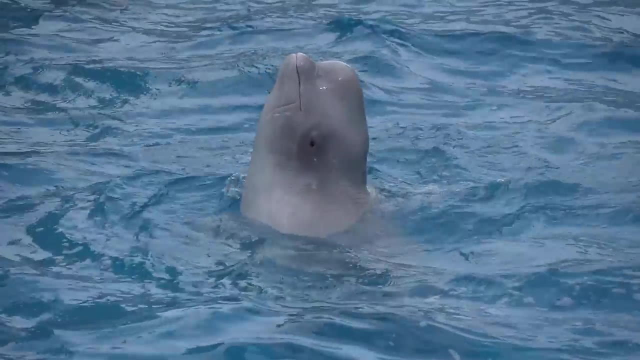 Black marlin and some sturgeons belong to this group. The ocean sunfish is the heaviest bony fish in the world and can weigh about 2,200 pounds. There are some animals that many people believe are fish, because these animals spend their lives in water too. but scientifically, 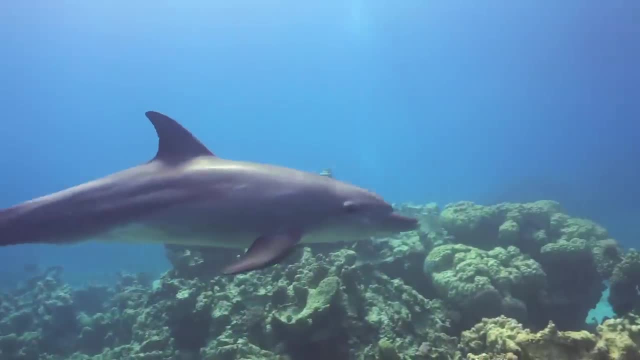 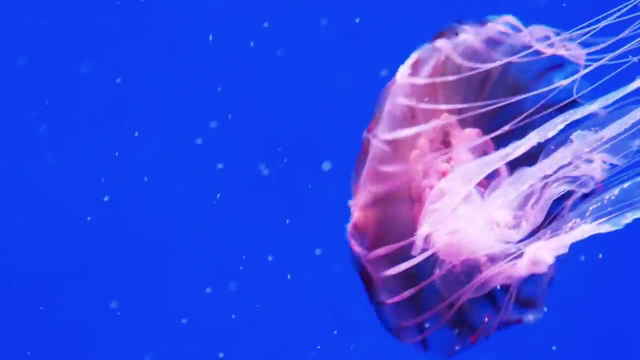 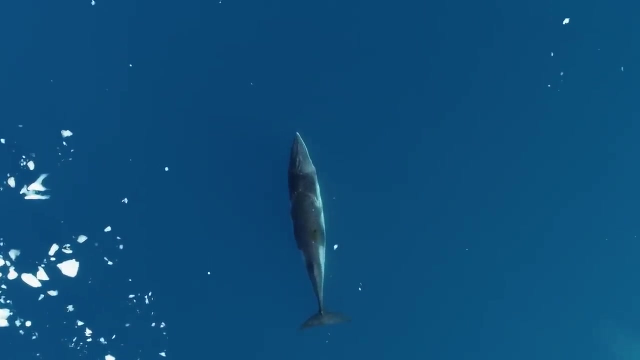 they are not fish. Whales, dolphins, octopus, starfish and jellyfish do not meet all the requirements needed to be called a fish, For example. dolphins and whales are warm-blooded. They don't have gills either. Instead, they have lungs, just like you. 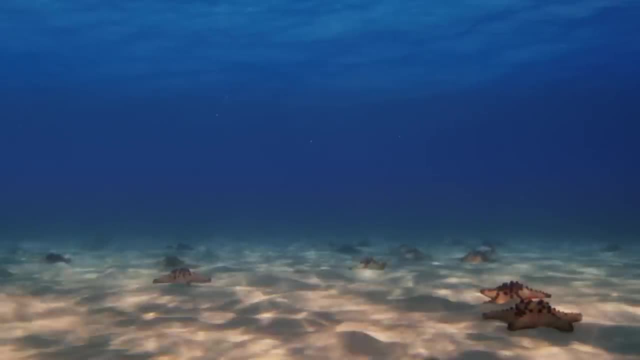 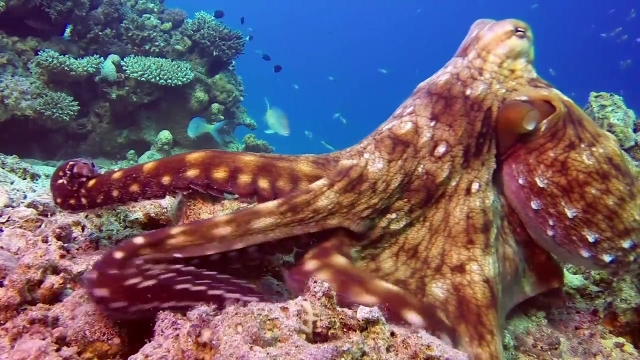 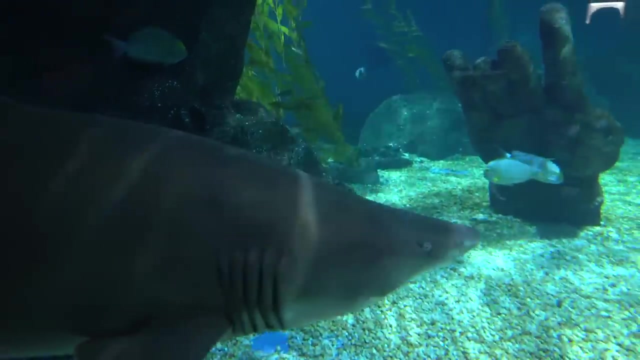 They are part of the mammal category. Starfish do not have fins or gills, and jellyfish and octopus do not have backbones or vertebrates, so they are not fish either. The biggest fish are sharks. Most sharks grow to about 40 feet and weigh an average of 20 tons or 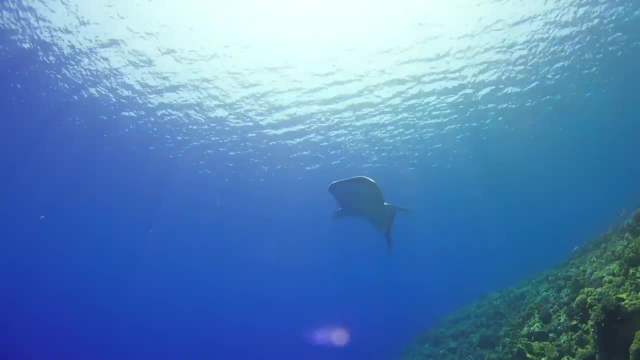 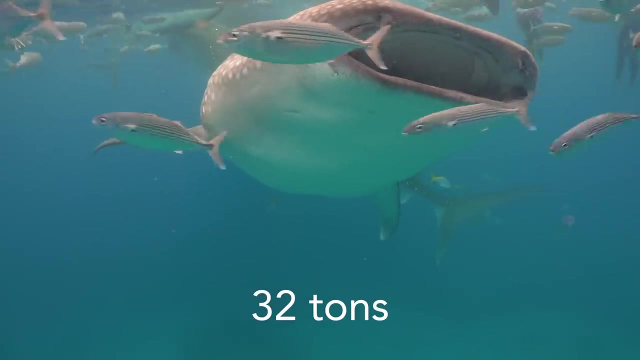 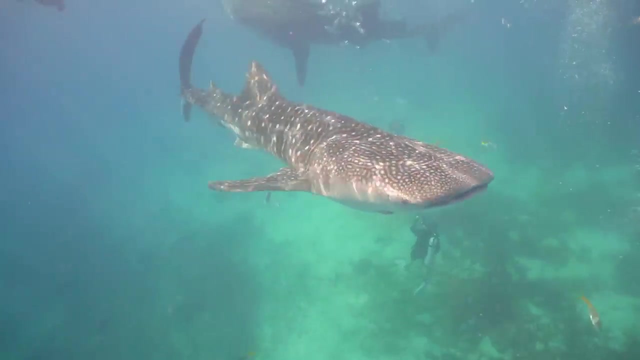 40,000 pounds. One type of shark, the whale shark, was the largest ever. measured at 60 feet long, It weighed 32 tons or 64,000 pounds. That might seem pretty terrifying, especially if you saw it swimming near you in the water. 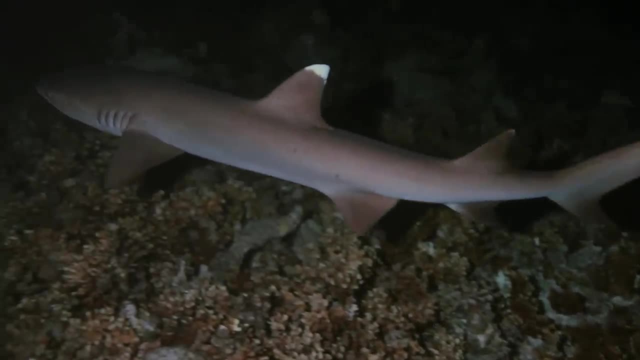 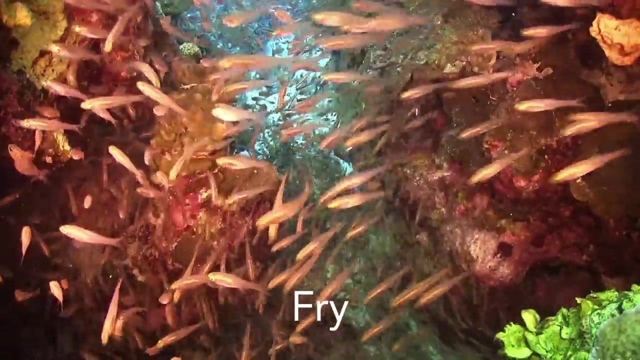 But sharks rarely attack humans. They would rather feed on their diet of other fish. A small fish is called a fry. It's not yet an adult, but it can feed itself. The smallest species of fish in the world has a long name. 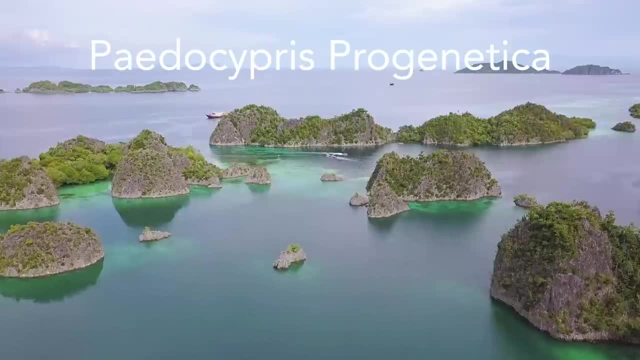 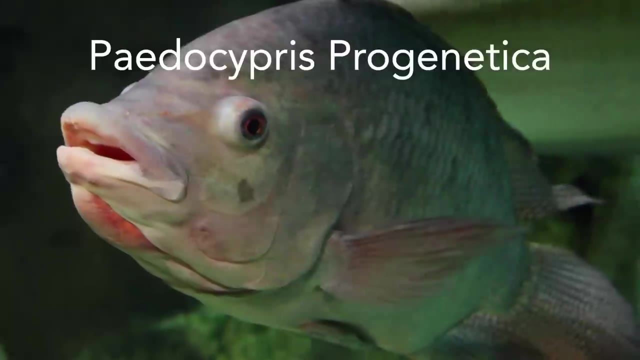 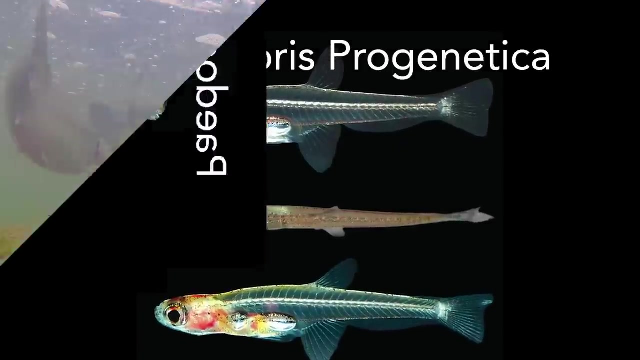 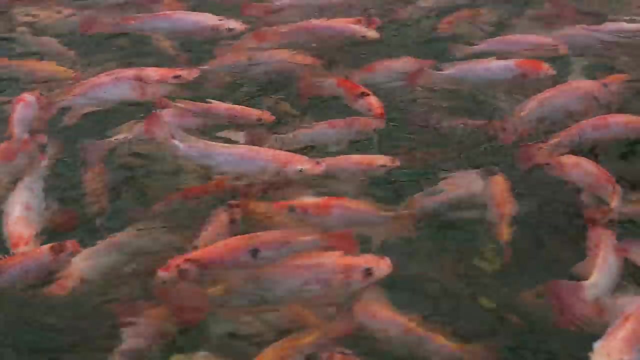 Pedocypris progenetica. It is found in the waters near Indonesia And measures only about one-third of an inch. It is a member of the carp family. It has a see-through body and a head unprotected by a skeleton. A common fish is a trout. A rainbow trout has beautifully colored skin which gives them their 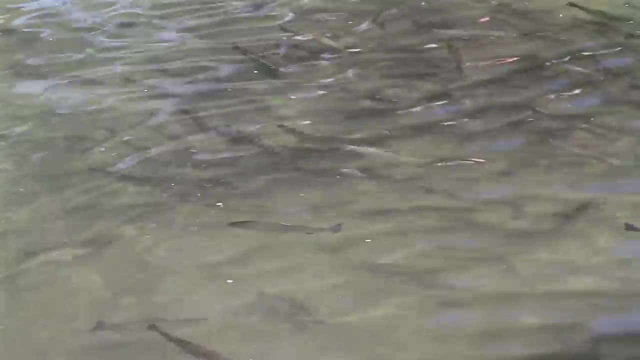 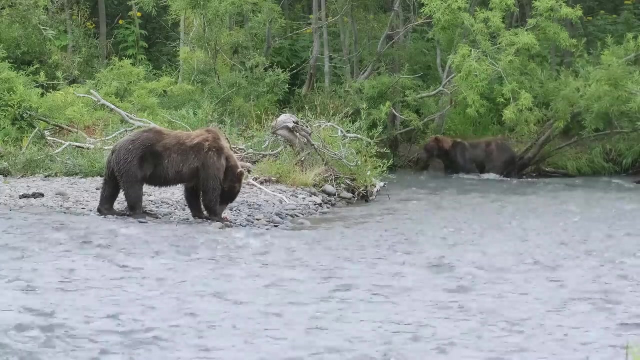 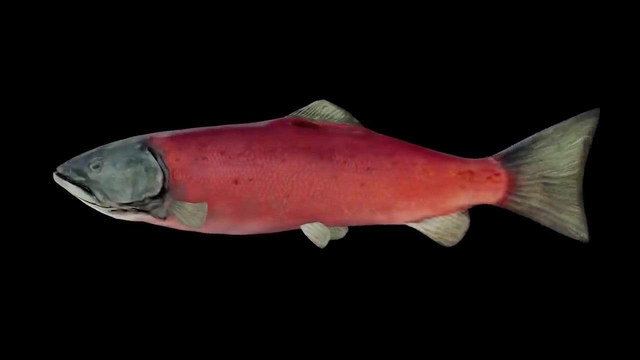 name. They are able to swim very quickly upstream. Trout are an important food source for humans, bears and other animals. They usually live in freshwater lakes and rivers. Salmon might be another fish you're familiar with. They are born in freshwater. 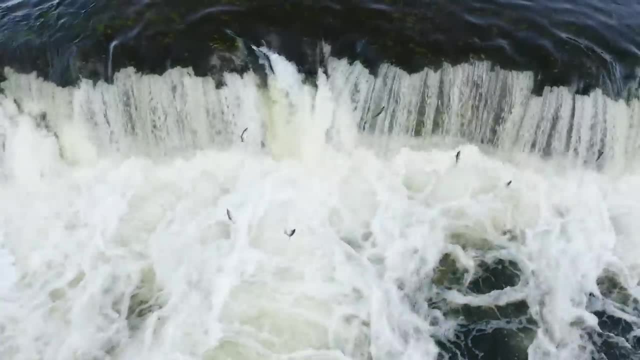 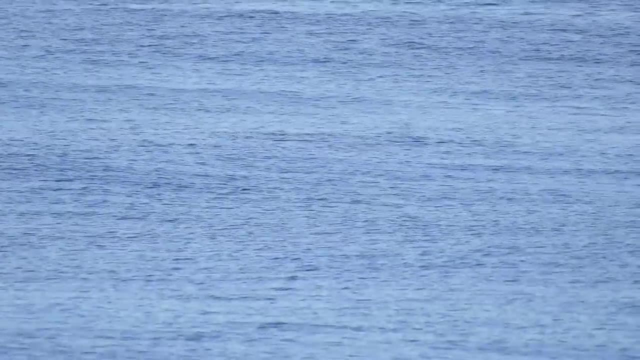 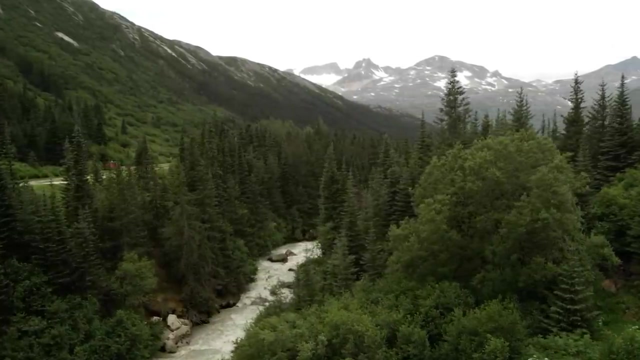 They travel all the way from streams and rivers to the ocean, A trip that can be hundreds of miles long. They might then travel another thousand miles in the ocean to get to their feeding ground. When it is time for them to make babies or reproduce, they 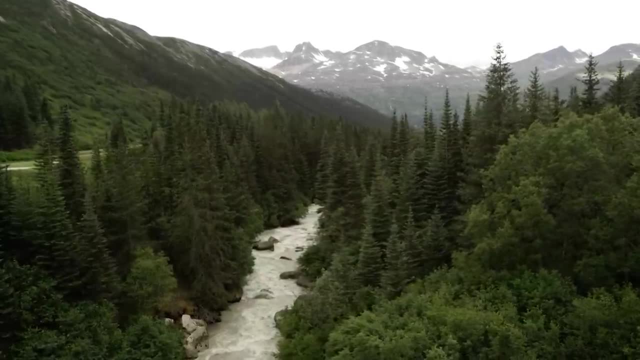 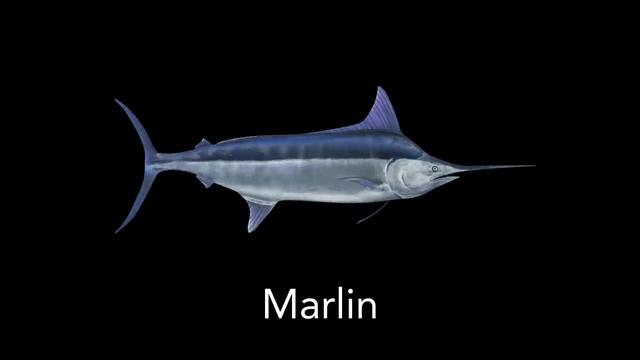 then return to freshwater, and often to the exact spot where they were born, Which is, though, usually far more infectious in their direct objeto: marlin. There are 10 different ocean species of marlin. These fish have long bodies and spear-like snouts. 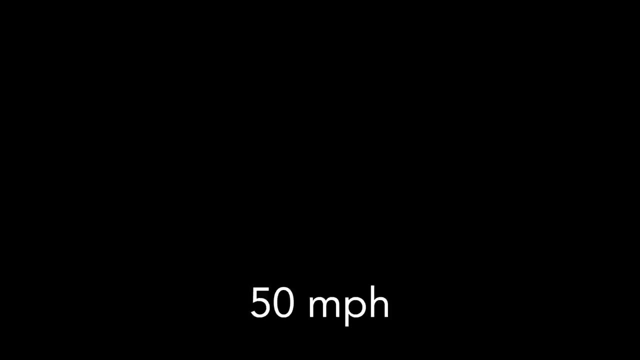 Marlin can swim up to 50 miles an hour And some can reach lengths of up to 16 feet and weigh 1800 pounds. That's 1,800 pounds. 2. An Endangered Vomiting, Geraldton nesteh, 1918- autopsy: A flat-rigid anglerfish are completely transparent. But it also lives back to feel better. Some fish can be so calm aboutμ. It can roam freelyrique and walk furiously in its natural habitat, never suffer an hassle of the life of a aikim ohonohika. There are swamps where the tideaire may qu BakeW teas written in and around you, and fish will not let itself slip by. 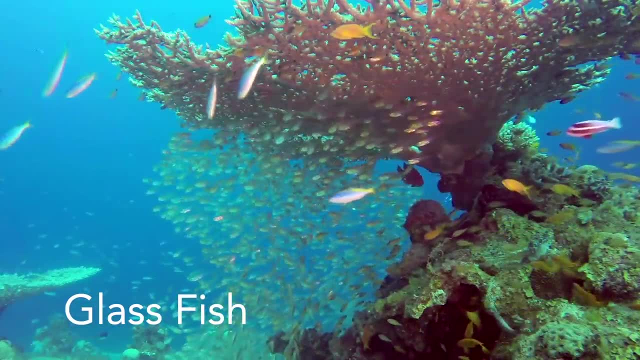 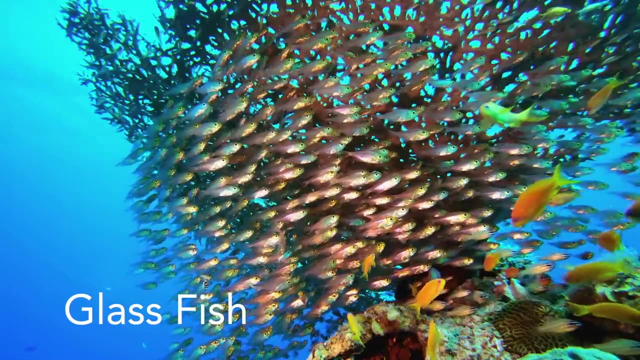 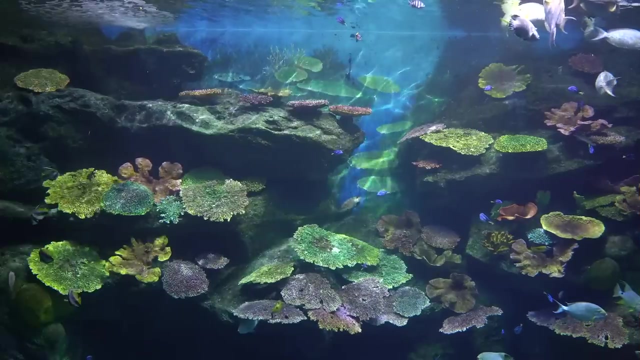 completely transparent, which means you can see all the way through them. They are great as pets, but they don't like to live alone. They do best when they are with their same species. Many people in the world depend on fish for food. Fish help our environment too. They are one of the biggest contributors of nutrients to the various ecosystems near them. Fish were the first animals on Earth with backbones, and they have existed for over 500 million years.